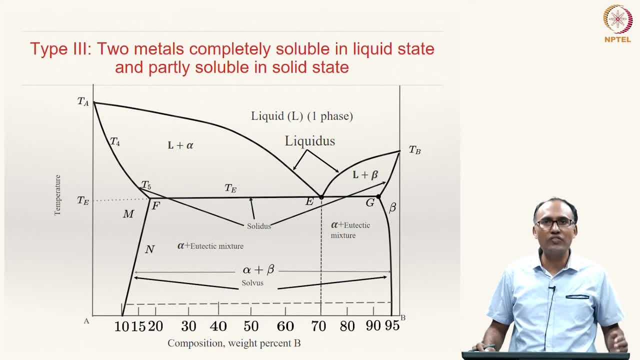 classified based on the solidification in the solid state. In the solid state they are completely insoluble. That means two materials, A and B, are completely insoluble in solid state, while they are completely soluble in liquid state. Now let us relax. 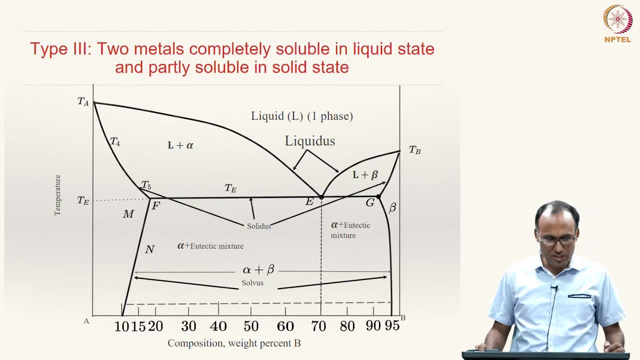 the constraint on the solubility in the solid state and instead of saying complete insolubility in solid state, let us say what happens if there is partial solubility in solid state while complete solubility is there in the liquid state. So that is why that is what we are. 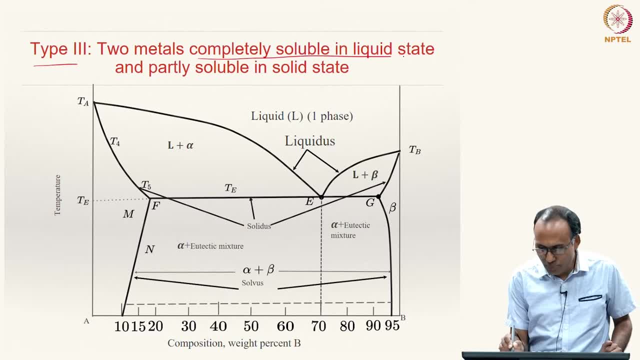 calling as type 3 alloys where you have where the two solubility are completely insoluble in liquid state and partially soluble in solid state. That means there is a solubility limit of A in B and B in A. So the phase diagram of such a system looks. 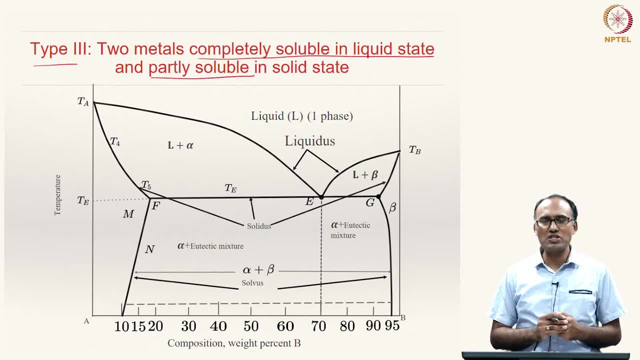 something like this: This phase diagram is a special case, or the type 2 alloy is a special case of this phase diagram. For instance, if you look at this phase diagram and move this point F and point G, If you move point G towards right and point F towards left, then it looks exactly similar. 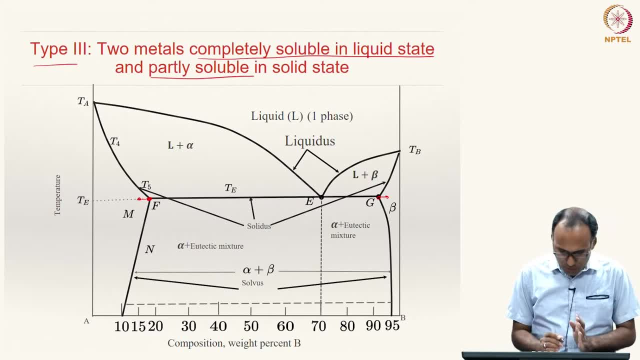 to our phase diagram of type 2 alloy right. Otherwise, if you look at the liquidus line- and this is our solidus line and up to in this region, it looks like your isomorphous alloys where they will meet at the some other point. So this situation is somewhere in. 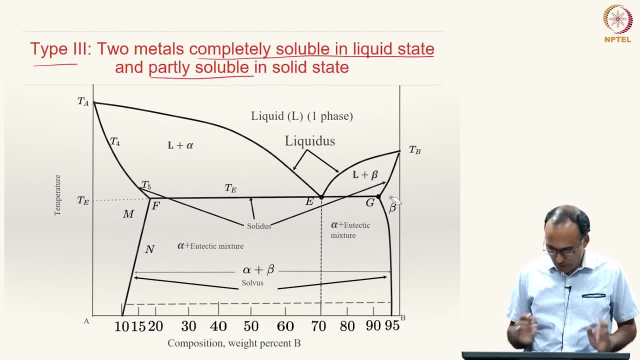 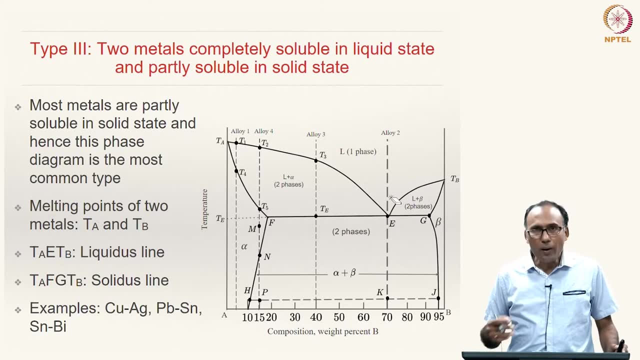 between the type 1 and type 2 alloys that we are seeing here. Okay, And this is an important alloy system to look at, because alloy system to look at because most metals are actually partly soluble in solid state, right? So this is the most common. 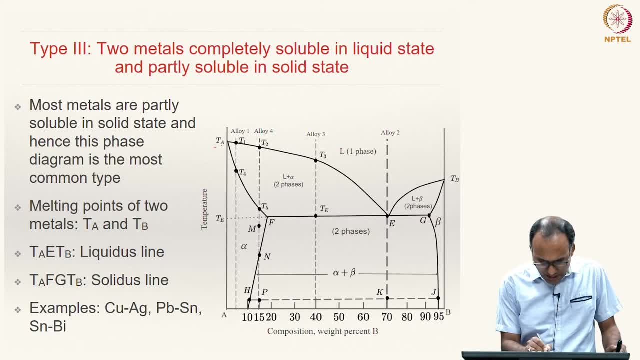 type of phase diagrams And you can clearly see here the T A and T B are the melting points of metals A and B and T A, E, T B. So that guy, Okay, Okay, That is our liquidus line, T A, E, T B, and the solidus line is T A, F, G, T B is our. 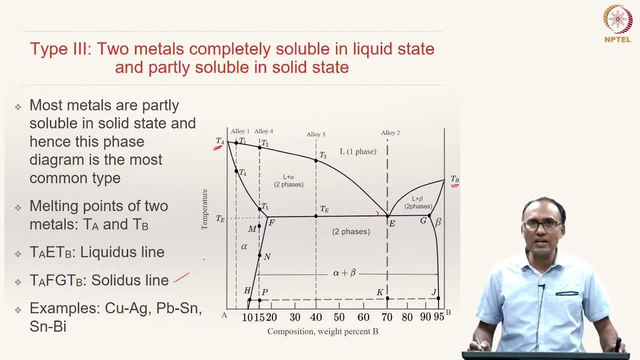 solidus line, And the typical examples of such a system, which has complete solubility in liquid state and partial solubility in solid state, are copper, silver, lead tin and tin bismuth. Alright, So here we again…. 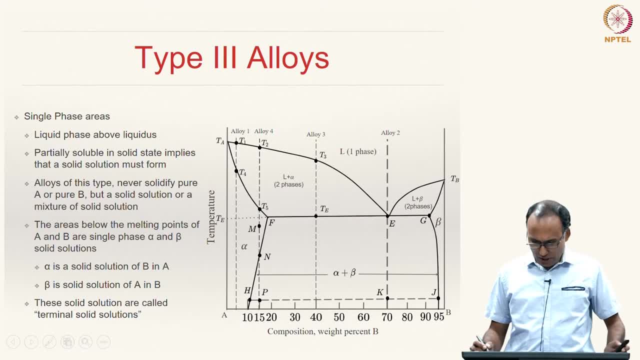 Okay, We have single-phase areas and two-phase areas, right? So here this is a single-phase area, and again you have another single-phase area here, another single-phase area here, and here you have a two-phase region, here two-phase region, and these also two-phase. 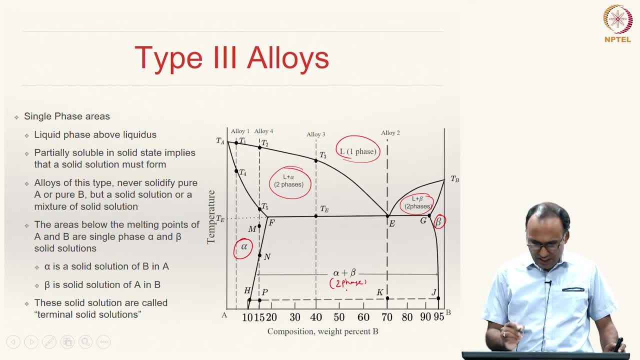 region. So, totally, you have three single-phase regions and three two-phase regions, And here please note that you have… you do not have pure solids. you have solid solution alpha and solid solution beta. Okay, So they… because there is a partial solubility of A. 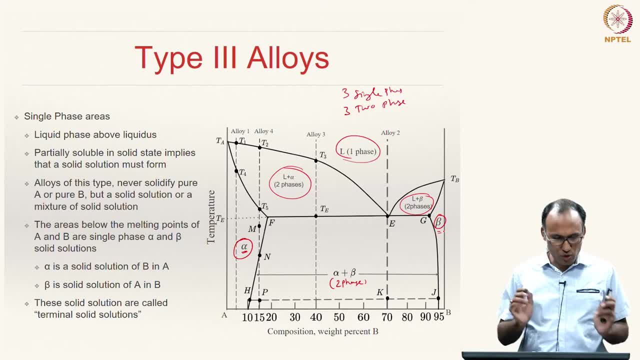 and B and B in A. they do not solidify pure solids. Alloys of this type never solidify pure A or pure B, but a solid solution or a mixture of solid solution will be formed. So the areas below the melting points of A and B are phases. So these are the phases. 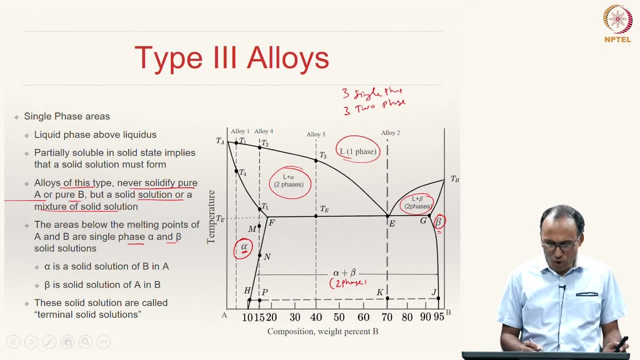 Or phase alpha, single-phase alpha and single-phase beta. usually they are called terminal solid solutions because they are towards the end, In between. also sometimes you may have phase diagrams between other compositions also you may have new phases, but the phases that 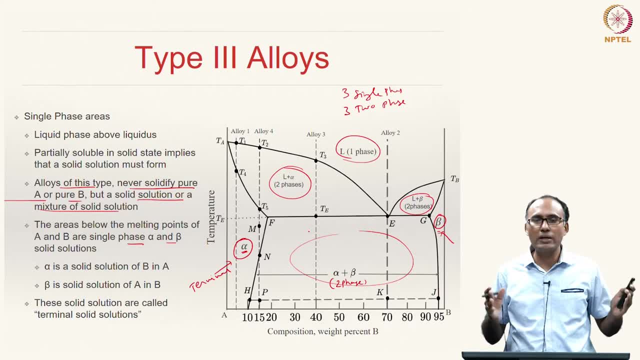 form towards the end of… very close to the pure solids are called terminal solid solutions. So here alpha is a solid solution which is rich in uranium. Okay, In A, So that means the solid solution of B. in A, So that means A is my solvent and 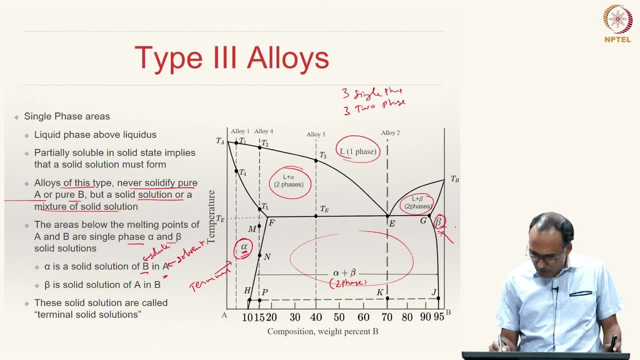 B is my solute in alpha. What is beta? Beta is a solid solution of A in B. That means B is my solvent and A is my solute, Right? So this is host and this is guest, Whereas in alpha, A is host and B is guest. Okay, And in between you have alpha plus beta. 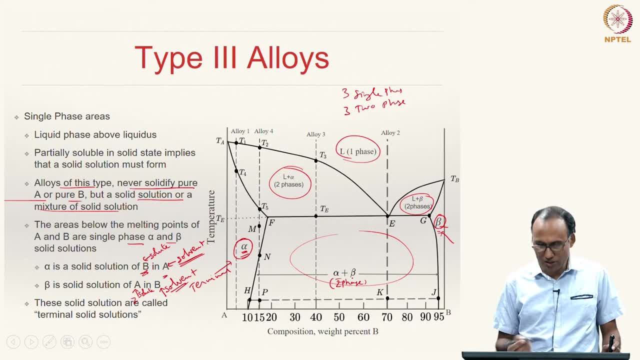 This is a two-phase region, So you can easily see how the two-phase regions are identified in this phase diagram, right? So, for instance, if you see this is a two-phase region, Why…? what are the two phases You? 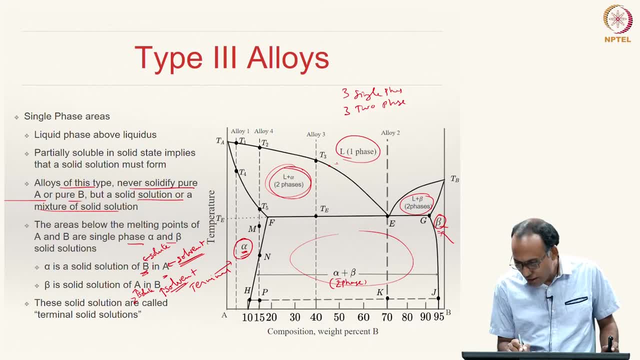 draw a tie line, You see that it is hitting this line. So, right to that, you have a liquid phase, and hence liquid phase is one of them. And here, left to this boundary, you have alpha, And hence these are the two phases. 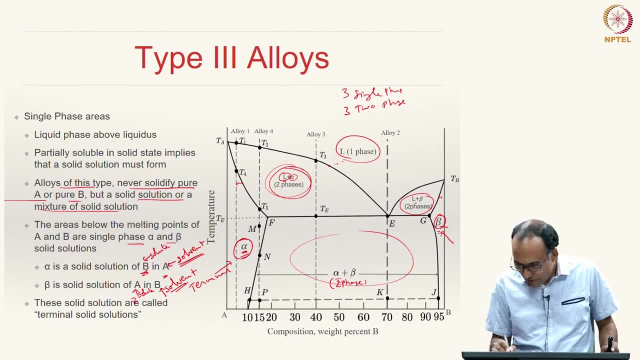 Similar here. right to this boundary you have beta. Left to that boundary you have liquid. So liquid plus beta. Here you have ruler fought or you have this level one side side. then you draw a line here and then you draw this line Right to this boundary. you have this. 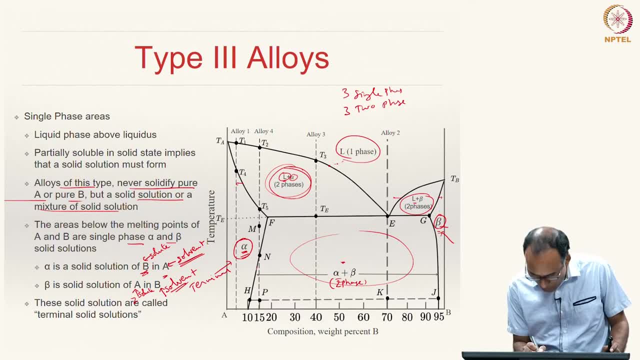 line Right to the finish, Right to you draw a line from here to there… Those are the two phases, a liquid, So liquid plus beta here in this region. left to this boundary, you have alpha, right to that boundary you have beta, and hence it is alpha plus beta. 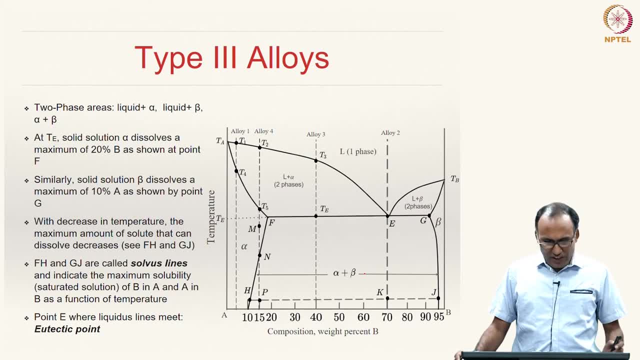 So the two phase areas are- we have actually already discussed liquid plus alpha, liquid plus beta and alpha plus beta. and at T e temperature. you can see, at this temperature there is a maximum solubility for this alpha right. The solid solution alpha dissolves a maximum of. 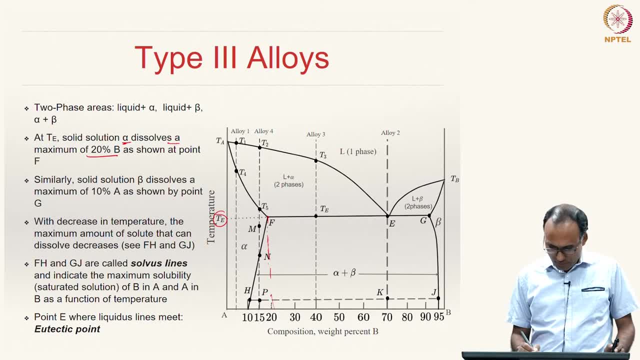 20 percent B. So this is the maximum solubility. right beyond that it cannot dissolve. So alpha has a maximum solubility of 20 percent of B in A. that happens only at T e temperature. at any other temperature it will have a much lower solubility, for instance at this temperature. 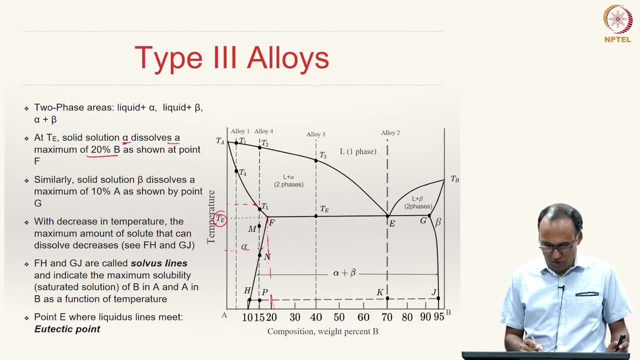 the solubility is only this much. at this temperature, the solubility is only this much. So the solubility changes. solubility changes. So the solubility changes as a function of temperature, as we have already seen in the. 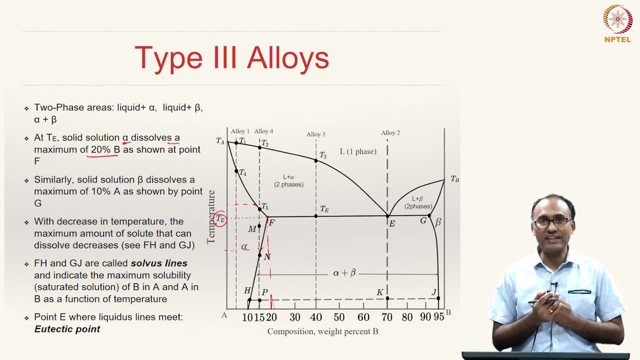 sugar water syrup, example that we have discussed in the very beginning of this module: right. Similarly, if you take beta at the same T e temperature, it has the maximum solubility of 10 percent of A. right, because it is 90, that means you have 10 percent A in B, which 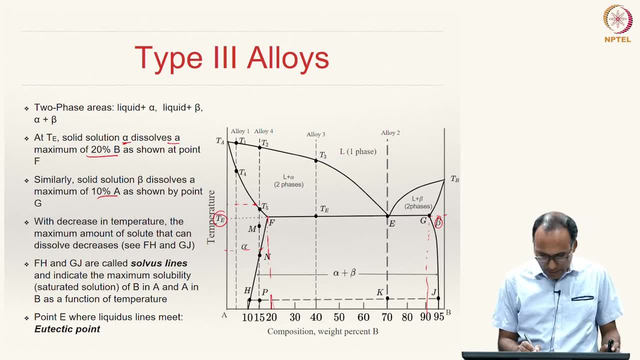 is described by point G and the maximum solubility of B in A is described by point F. So the solubility of B in A is described by point G and the maximum solubility of B in A is described by point F. 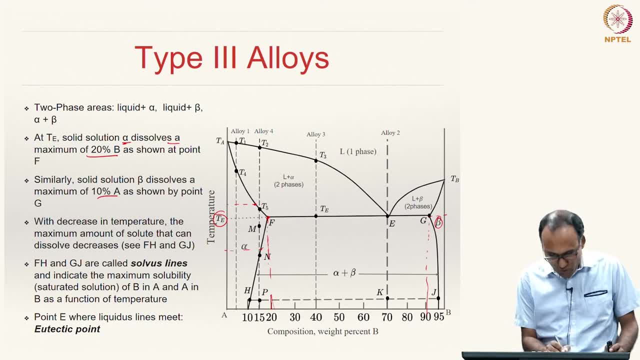 And with decrease, further decrease in temperature, the maximum amount of solute that can dissolve decreases. right, because the solubility is decreasing with decreasing temperature. in both the cases, all right. And here the lines F, H and G J. So this is our F H line and 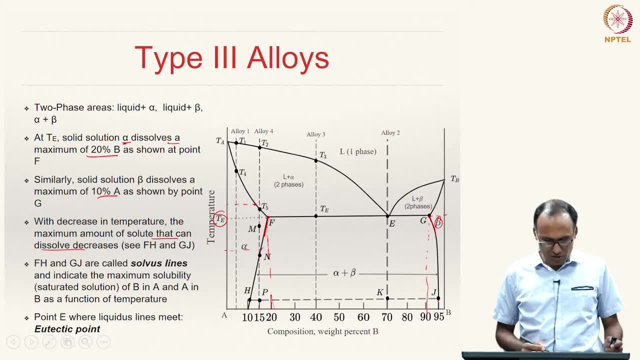 this is our G J line and these two lines represent decrease in the solubility of the solubility of the solute atoms as you decrease the temperature. And these two lines are called solubility. They indicate the maximum solubility of B in A and A in B as a function of temperature. 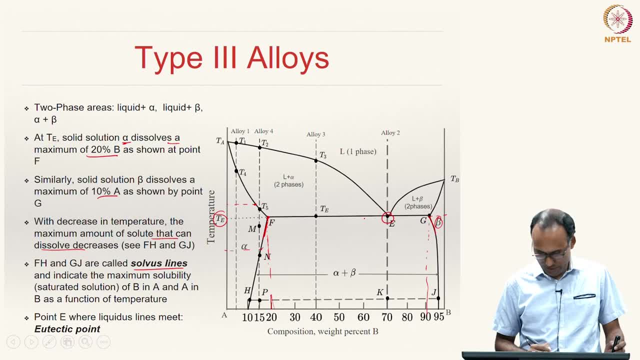 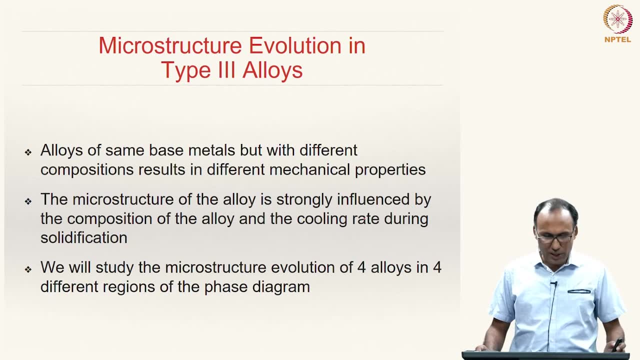 and point E is again your eutectic temperature or eutectic point. all right, So how does this microstructure look like is something that we will look at. So we need to certain interesting aspects of these type of alloys, So alloys of same base metals. 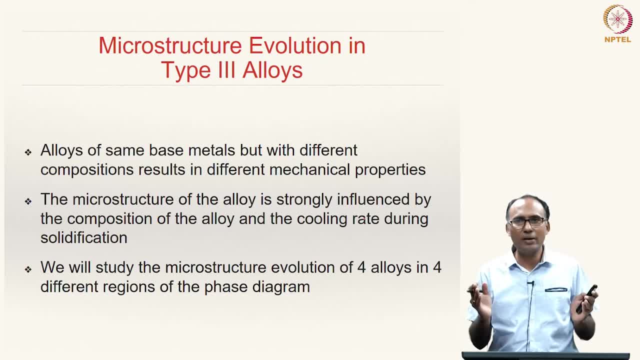 but with different compositions. So that means A and B are the same, but different compositions will result in different mechanical properties, and that is the reason why we need to study their microstructures, because the microstructure is going to be strongly influenced by the composition of the alloy and the cooling rate during the solidification. 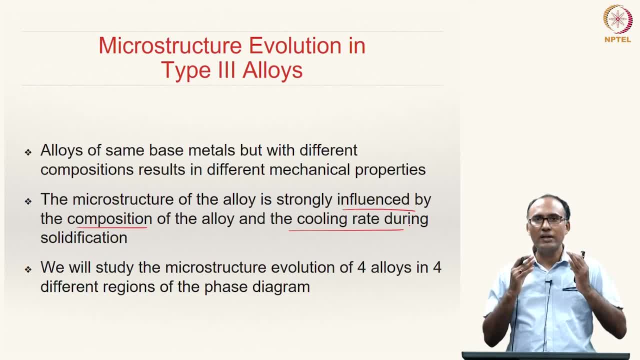 However, in this module we are not looking at cooling rate. we are assuming that the cooling is done and at a sufficiently small rate, which means the equilibrium cooling is done. So effect of cooling rate will not be discussed in this module. it will be discussed at a 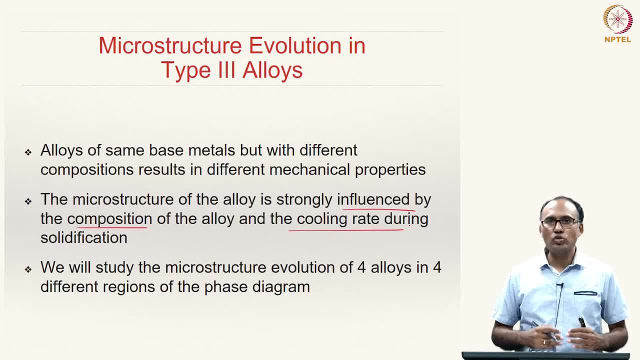 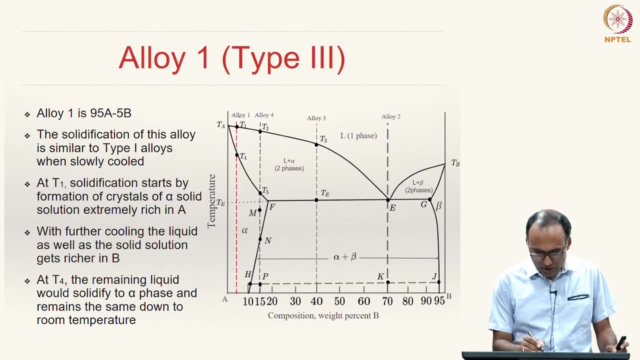 later stage. So the key to the properties of different alloys is the microstructure, and hence we will study the evolution of the microstructure for four different compositions or four alloys in four different regions of the phase diagram. So this is alloy 1, alloy 2, alloy 3,, alloy 4.. We could also have another alloy in this. 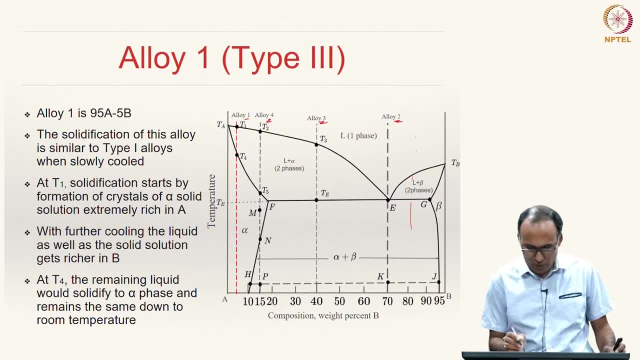 region, but that will be similar to alloy 1 or alloy 4.. So that is why we are studying these four classifications. Now let us look at alloy 1,. alloy 1 is 5B- 95A, this is say 5 percent B and 95 percent. 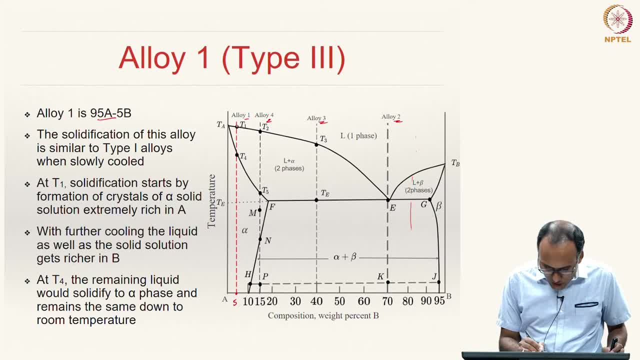 A. So the solidification of this metal starts, this alloy, starts at temperature T 1 and ends at temperature T 4, and so it enters the two phase region. then you will have liquid plus solid. that solid will be alpha solid solution, and when it comes down it again enters from the 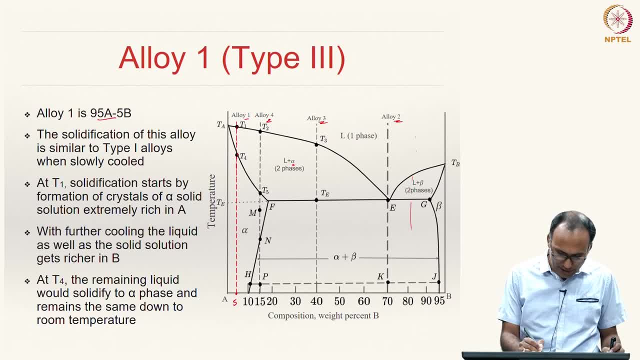 two phase region. all the solidification, all the liquid would have transformed to alpha and then you will only have alpha. So this alloy microstructure is very much similar to the case of isomorphous alloys that we have looked at, wherein the liquid 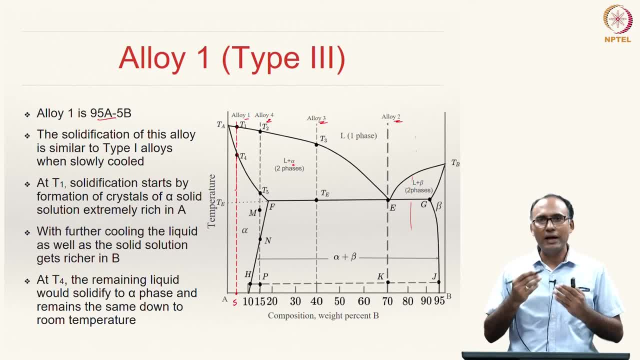 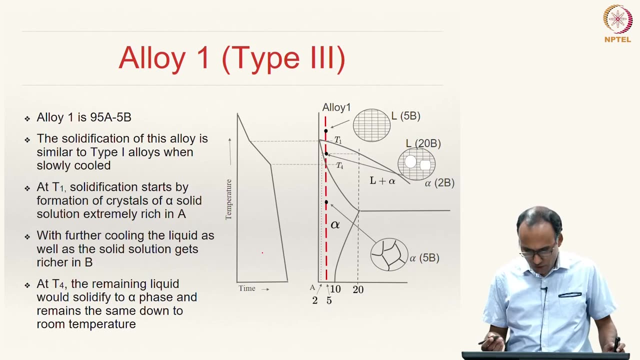 starts solidifying at temperature and then ends at another temperature when all the liquid would have transformed to another solid phase, single phase. So this is very similar to our isomorphous alloy microstructure. So you have a liquid and then up to somewhere. 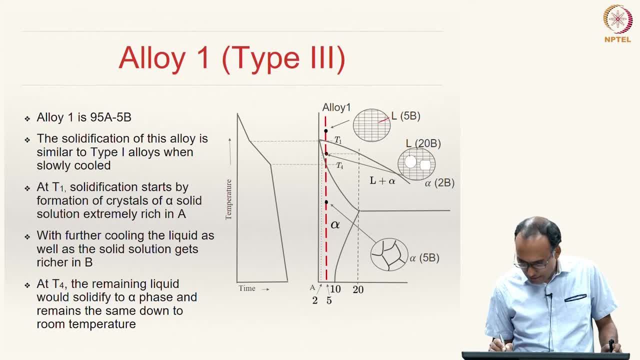 in between, you will have solidification happening, and this is alpha and this is alpha grains, and by the time it reaches T 4, entire solidification would have finished. As you are coming down, all that happens is the alloy composition is phi b, but everywhere you have the solubility at each and every temperature. 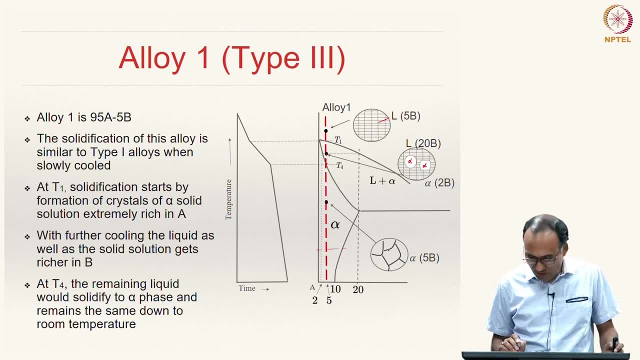 is much larger, So it is actually not under saturated and hence nothing will happen. So the alpha will simply this: as you are cooling down, it simply reduces the. it reduces the sensible heat, Basically the temperature of the solid reduces, nothing else happens. 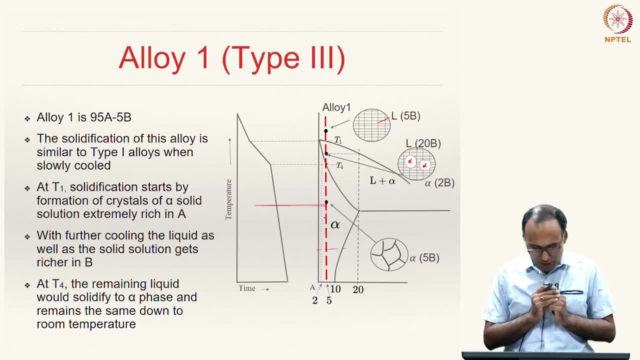 as far as the microstructure change is concerned. So it is very similar to alloys. So this is solubility. The purpose of solubility is there. This is a히, since we have the يso, that is the a히 yourselves, so we can substitute that. 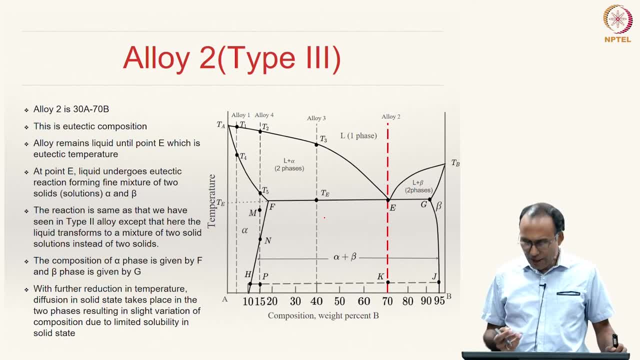 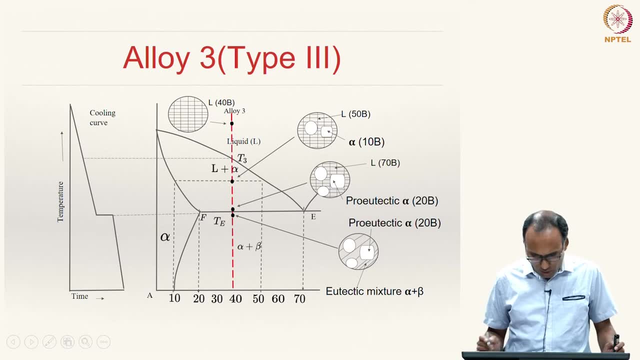 let us look at alloy2.. again, alloy2 is our eutectic alloy because it is an eutectic composition. Let us look at the microstructure. So at this position you have, everything is liquid. And now let us at T3, the solidification starts and on the left hand side we are showing. 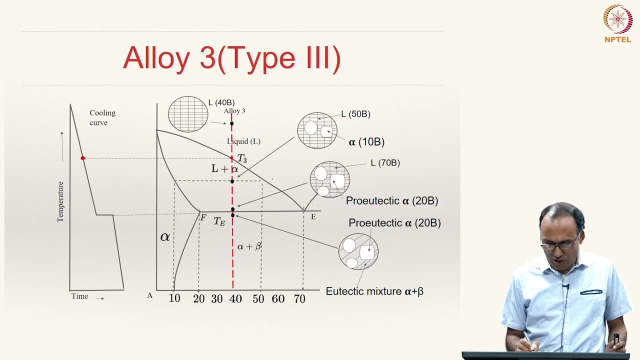 the cooling curve. So here the solidification starts at this point, and then, as we are cooling, cooling down, the liquid starts becoming richer in B and alpha starts. So the liquid solidifies into not pure A, but into a solid solution of type alpha, which means solid solution. 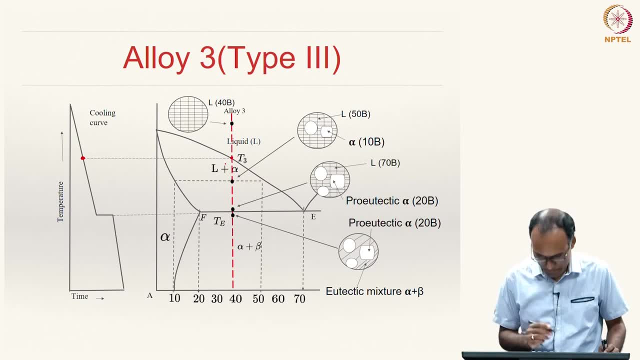 of B in A. So alpha is a solid solution which is rich in A, So it solidifies into alpha. So alpha crystals will be formed and they grow over the time, And then the remaining liquid. so by the time you are here you have some amount of liquid and remaining is pro-eutectic. 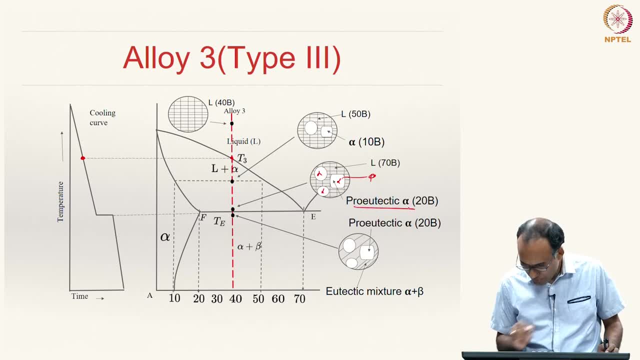 alpha, So it is called primary alpha or pro-eutectic alpha. So if you look at the composition, so like draw the tie line. So here it is 20B. So that is the composition of pro-eutectic. 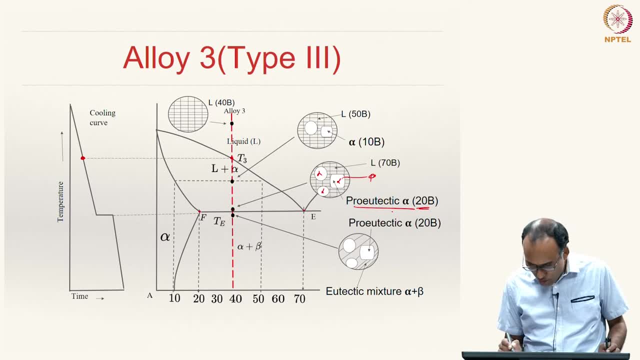 alpha and the remaining liquid solution composition is equal to eutectic composition. that is 20B Here 30B, So the liquid is 70B. So not 30B, 70B. That means that is our eutectic. 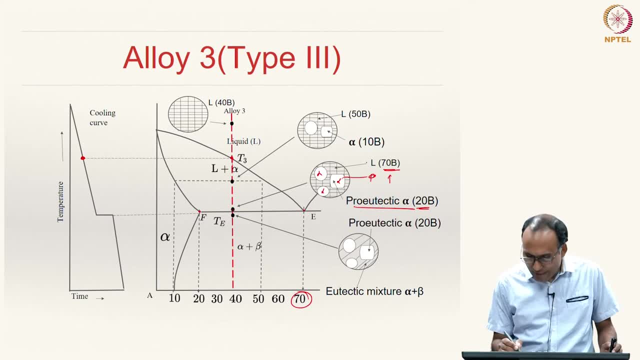 composition. in this particular system, Since the remaining liquid has reached the eutectic composition and the temperature is eutectic temperature, what should happen? The remaining liquid should go through a eutectic reaction. And when it goes through a eutectic reaction, 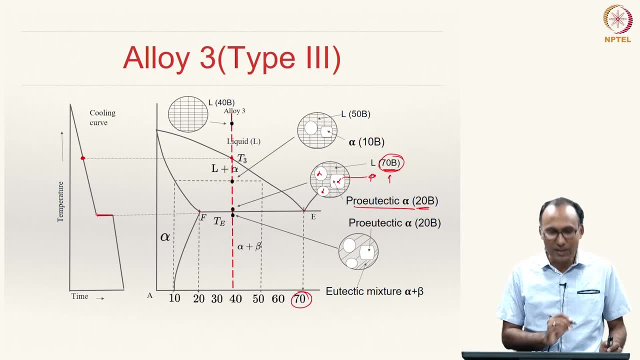 that happens at constant temperature. That is why you see a constant line, because the remaining liquid, up to here, the liquid is crystallizing solidly, So the solid alpha, and then, at this point, the remaining liquid has reached the eutectic. 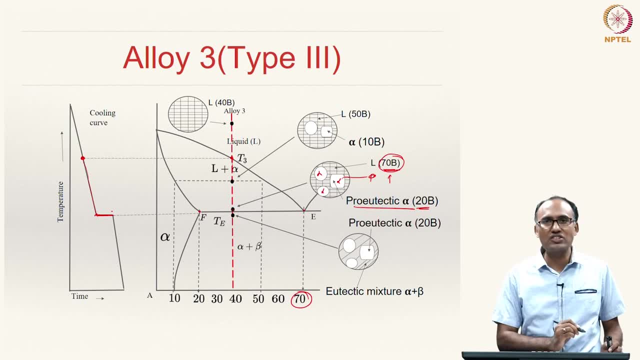 composition and eutectic temperature, And hence at constant temperature, the solidification happens. And the solidification results in formation of two solids, a liquid transforming to two solids. Here the two solids will be two solid solutions, So alternate layers. 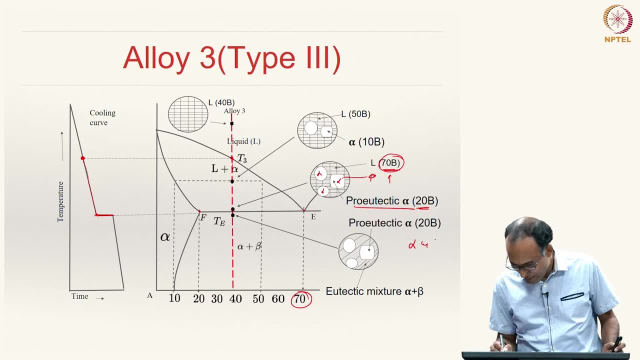 of alpha and beta, So the two phases will be alpha and beta And it becomes an alternate layers of alpha and beta. So let us say: this is alpha and that is beta, So this is alpha, beta, alpha, beta and so on. So the final microstructure will be a pro-eutectic alpha. 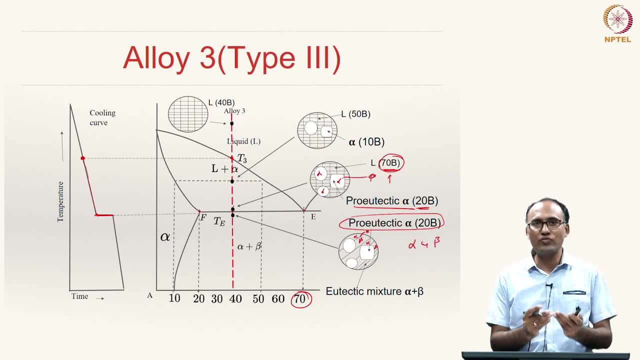 which has been formed before, which has been crystallized from the liquid solution before the eutectic reaction took place, And the remaining liquid transforming to alternate layers of alpha and beta. Here we are forming alpha and beta because pure solid A and solid. 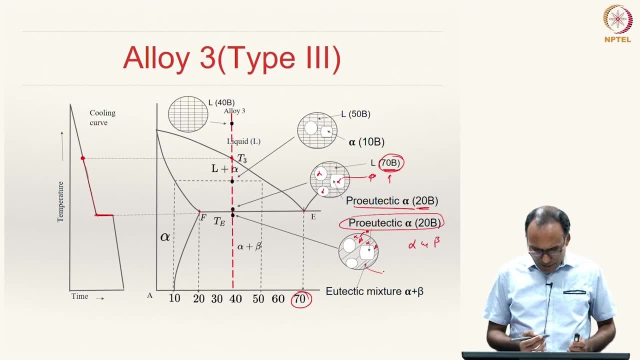 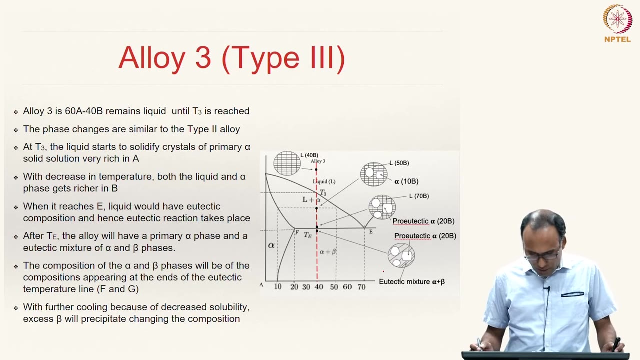 B cannot form because there is some partial solubility And you can also calculate all the weight fractions based on the discussions that we have discussed. So this is what we have so far. we had so far on different other systems. Now let us look at alloy-3.. Alloy-3, so here again, sorry, Alloy-3 is also pretty straight. 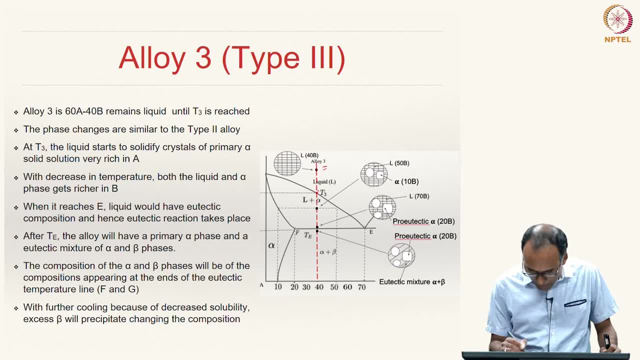 forward. You have a complete liquid solution at time. temperature, t 3, small grains of alpha start solidifying And you see, somewhere in between you will have you draw a tie line and you see that it is 50B. So the liquid composition will be 50B. 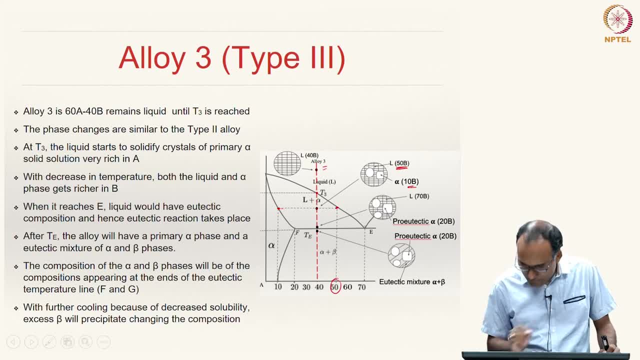 and solid will be. that is, alpha composition will be 10B And if you further cool it down just above the at this point on this line, then the liquid composition will be 70B. So that means you take the composition and solid will be 20B. periodic alpha will be 20B. So 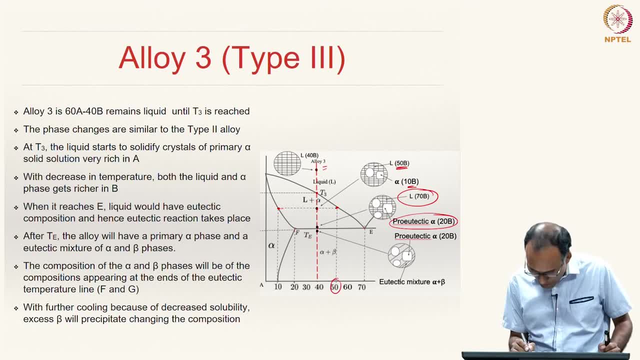 whatever remaining liquid, whatever is the weight fraction. what is the weight fraction of this liquid? The weight fraction of the liquid will be this distance divided by the total distance. This distance is weight fraction of liquid. here, at this position, is 20 divided by 50, because 20 minus 50 is 70 is 50, that is equal to 2 by 5, that is equal to 40 percent. 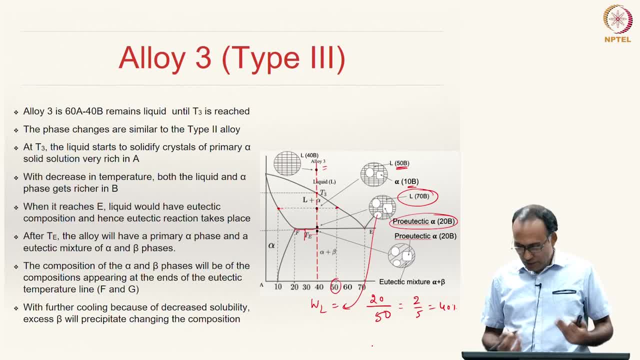 So the 40 percent liquid would transform to eutectic mixture of alpha and beta. So somewhere here, if you look at the microstructure, you have pro eutectic alpha, which is 20B, and eutectic mixture of alpha. 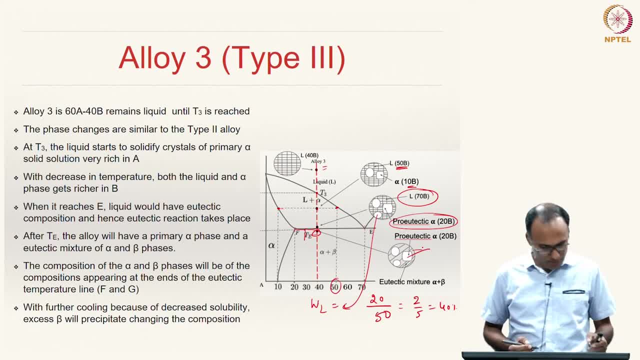 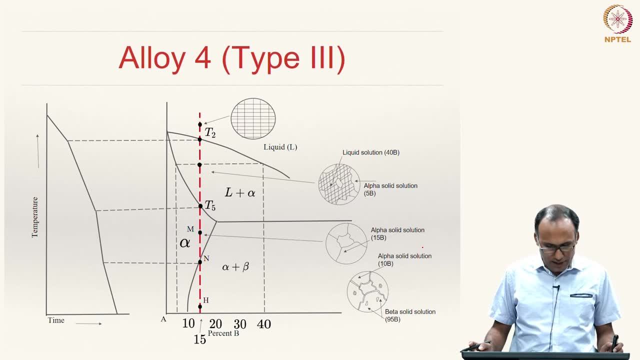 and beta. Now let us look at alloy 4, which is an interesting alloy here. Now let us first: at this position everything is liquid and at temperature T2, the liquid starts solidifying, So that means initial alpha phase starts happening. 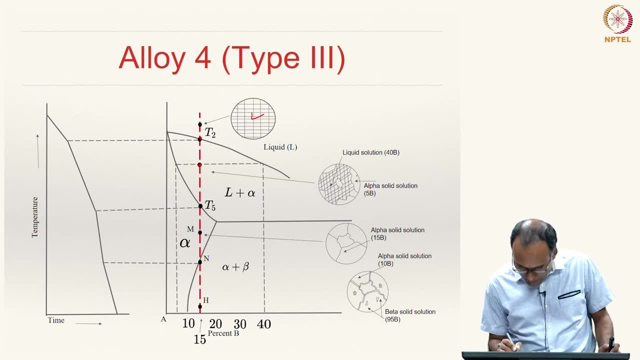 And then, at some intermediate temperature, we are seeing the alpha solid solution. this is alpha, this is alpha, alpha, alpha, alpha, alpha and the remaining liquid. And here, if you see, the composition of alpha is 5B and the remaining is liquid. liquid will be this: 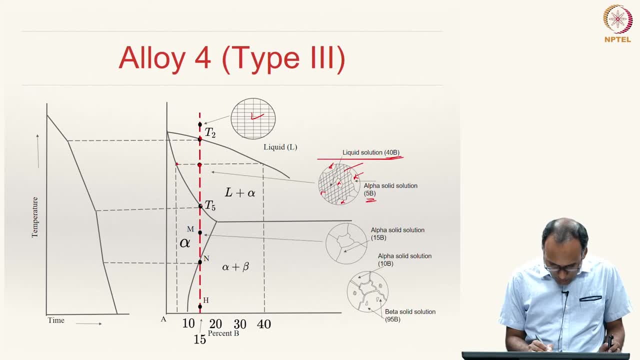 is 40B, And now, the moment you reach temperature T5, all the liquid would have transformed to solid alpha. All the liquid would have transformed to solid alpha. Right, So that is like our isomorphous alloys. So at this position you will have complete. 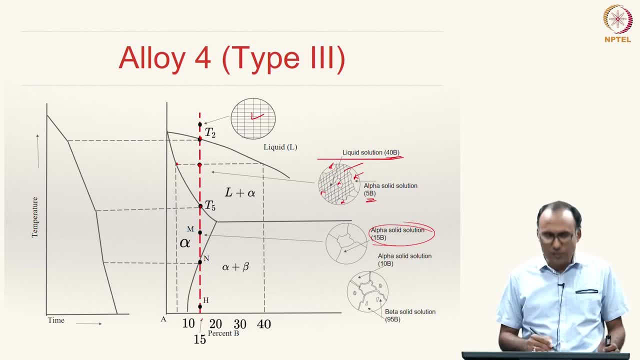 alpha, And here we have started with 15 percent B. So all the alpha would have transformed to 15B. And if you further cool it down, what happens at N? when you are further cooling it down here, the moment it reaches point N, the solidification, the solubility limit, 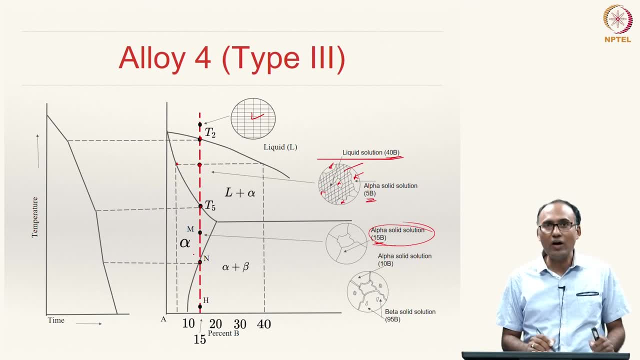 has reached saturated. So that means at N it can have 15 percent B. So we already have 15 percent B, So that is saturated. The moment you come below, if you cool it down below this temperature point N, what happens? The solubility limit is only this. 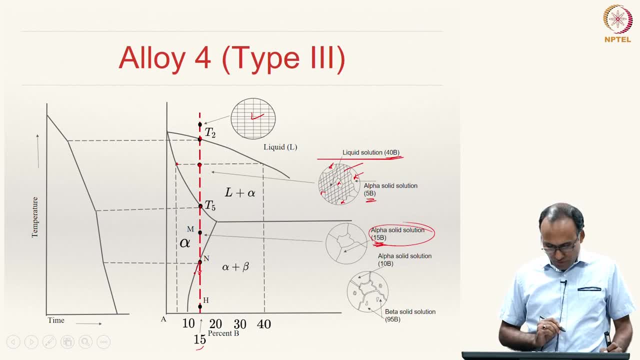 much, but your composition has 15 percent B. So let us say you are looking at H, point H, Your composition is having 15 percent B, but your solubility limit says that if you are less than 15 percent, what you want to use H is less than 15 percent B if you have. 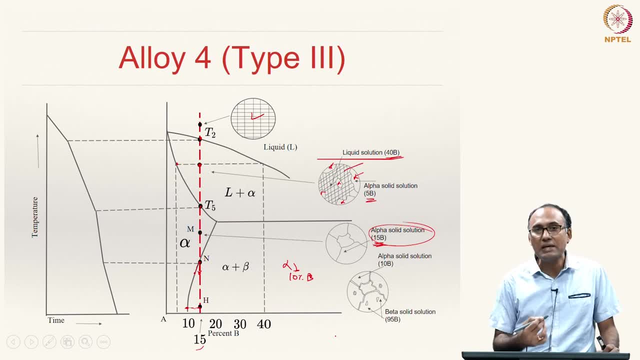 15 percent H won't be for the next fixed alpha. Then you would have this fourth part of the appears exactly like what you do, that is, like that is a 1 to the 2 of M. Yes, Hence it comes out as solid solution beta, and this solid solution beta is actually dispersed. 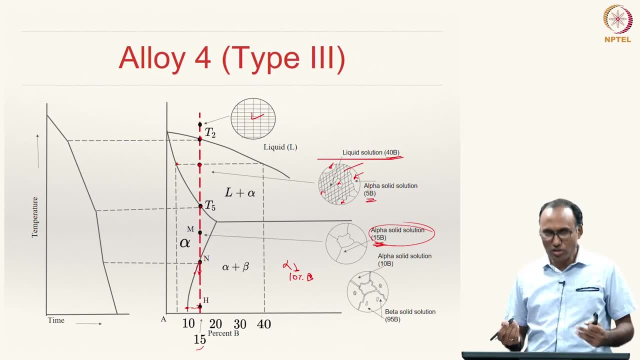 everywhere, throughout the alpha matrix. So what will be the microstructure? what will be the weight fraction of that beta? that will be. So, if you draw a straight line, tie line, it is in the two phase region. this line hits the g, h, g, j line at 95 b, and hence the composition. 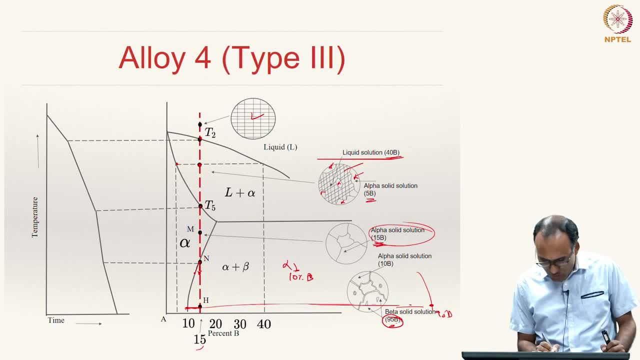 of beta solid solution will be 95 b and the weight fraction will be very small. only this much is the weight fraction of beta and this beta is usually found. this beta solid solution comes out. the b additional b that is sitting in alpha comes out as beta solid solution. 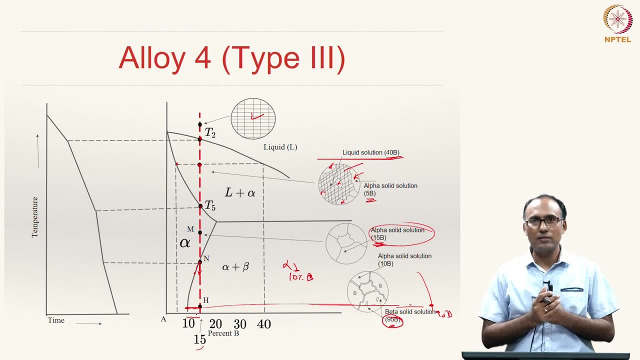 and that is randomly distributed throughout the matrix and preferentially along the grain boundaries. So these are our grain boundaries, these are our alpha grain boundaries. you may have beta sitting, So you can see that beta solid solution is dispersed throughout the grain boundaries and also in the matrix. So here, because of the limited solubility, as you are cooling down, 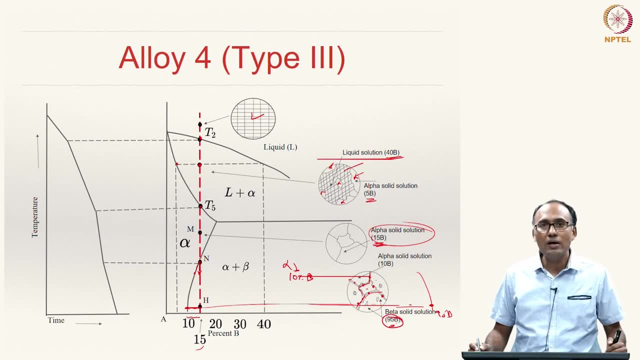 there is something more happening to the microstructure, So the still there is some events taking place because of the limited solubility and hence the position of the solvus line is also an important aspect to be paid attention to right And please note that in this particular system your after t 5 you are under single phase. 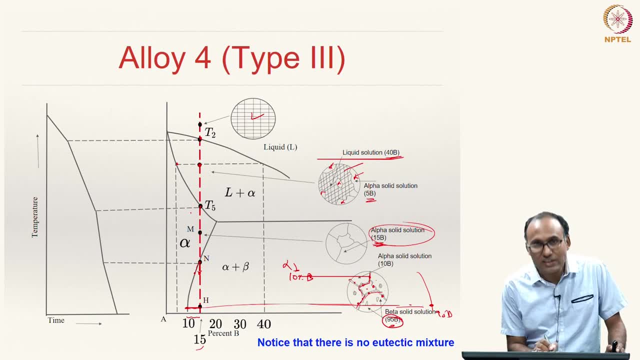 region, since you have in a single phase region. you do not have a tie line concept and does not. although you are crossing through the temperature T e, there is no liquid anymore. everything is solid first of all and there is no reaction taking place. So that means 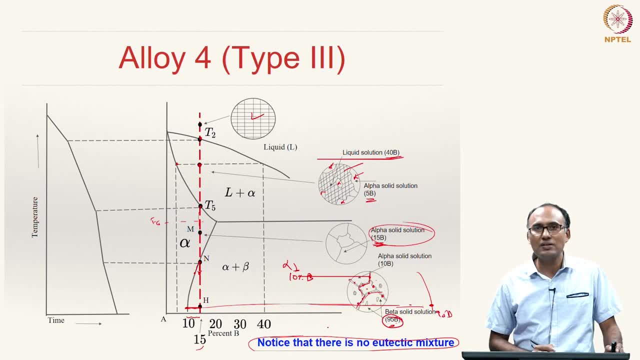 you do not see eutectic mixture in this particular mic micro structure. Thank you. So, although there are several alloys which will form eutectic mixture, but this particular composition is not going to give you any eutectic mixture. 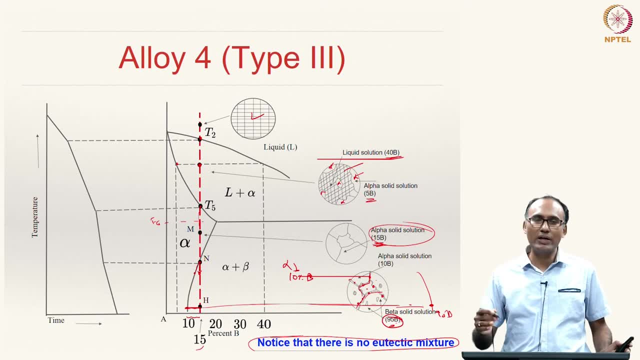 In that sense alloy 4's microstructure is very different from alloy 2 and alloy 3, also from alloy 1.. Alloy 1 is like very simple microstructure, like isomorphous alloys, but alloy 4 is really interesting because it is going through. please note that here it is again going from a single. 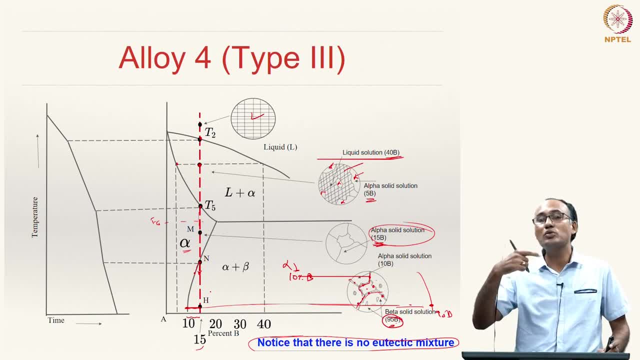 phase region to two phase region, without actually going through any reaction, but just by giving out B from the excess B. So because of the over saturation, of the over saturation of alpha solid solution with B, the additional B has to come out and that comes out as beta. 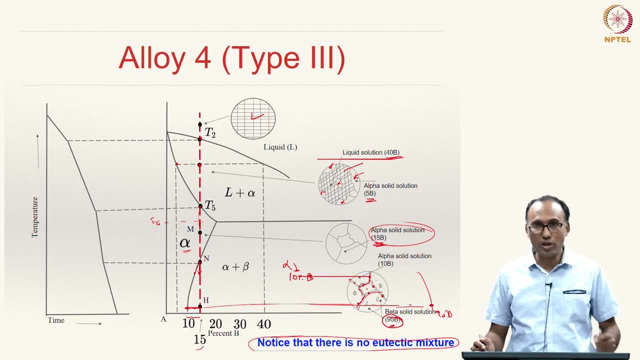 solid solution and that will be dispersed uniformly within the matrix. So you are actually going from a liquid solution single phase region into a two phase region- liquid. So you are actually going from a liquid solution single phase region- alpha plus alpha- into another single phase region- alpha, and again entering a two phase region alpha plus beta. 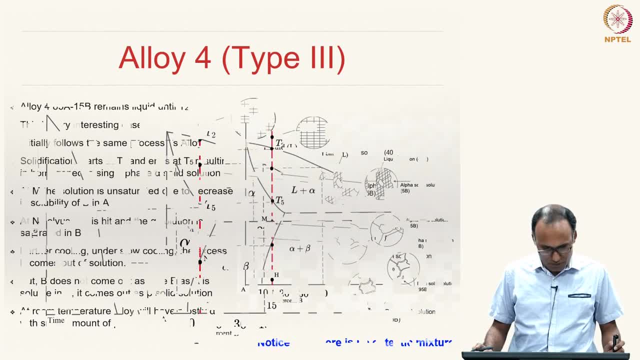 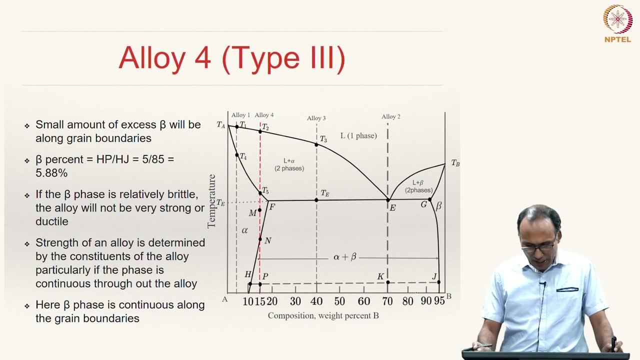 So that is about alloy 4, so the microstructure looks something like this and we can also, in the two phase region, we can calculate what is the weight fraction of beta. So we can see that if you are drawing this line, this, the weight fraction of beta, will. 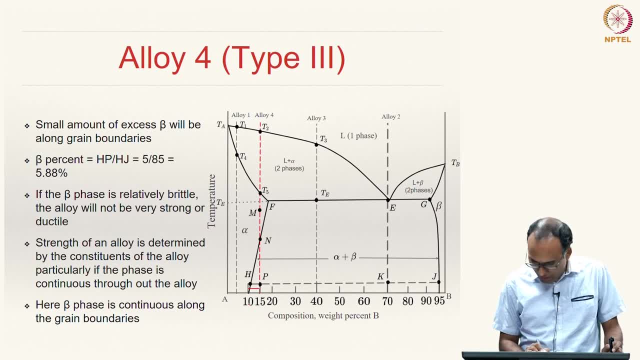 be H p divided by H j. H p will be 5 divided by H j is about 85. That will be about 5.88 percent when you are looking at the alloy 4 and if you please note that, if the beta phase happens to be a relatively brittle phase, 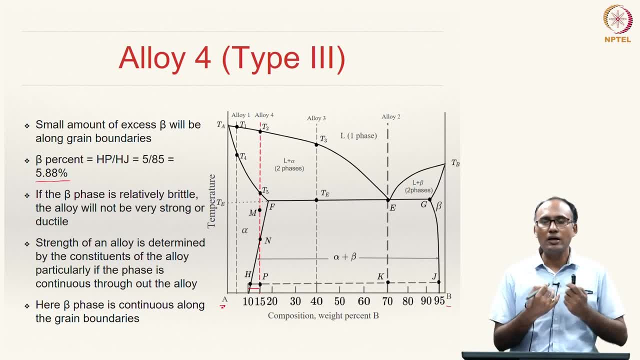 Let us say that the beta element A and B are there. let us say A is a soft version and B is a brittle phase. and if the beta phase is relatively brittle, then what happens is because of the distribution of this beta phase throughout the alpha. 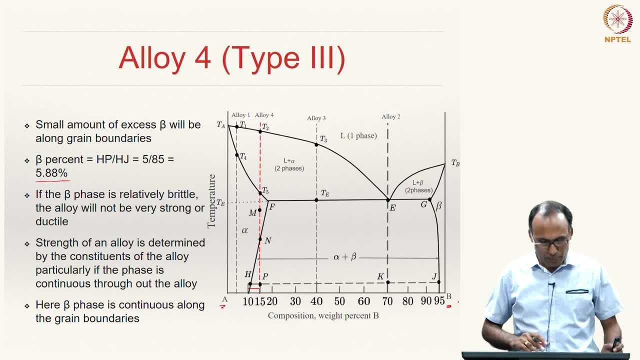 So you can see that. So in the case of the beta microstructure, this beta brittle phase can actually make the material vulnerable for failure, because it may not. because of its brittleness, it may not be very strong or ductile. 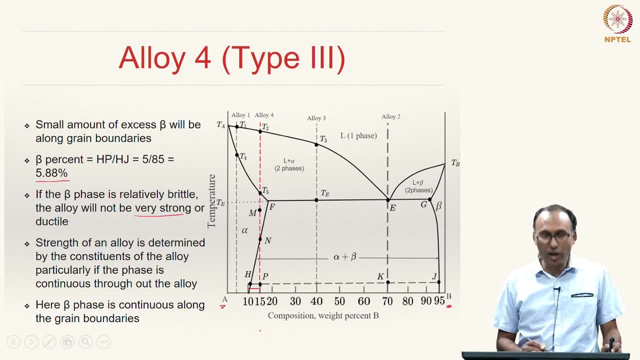 And so from this particular alloy thing, alloy composition, we can understand that the microstructure plays a critical role in understanding the strength of an alloy. So the strength of an alloy, as we have discussed, that is determined by constituents of the alloy. 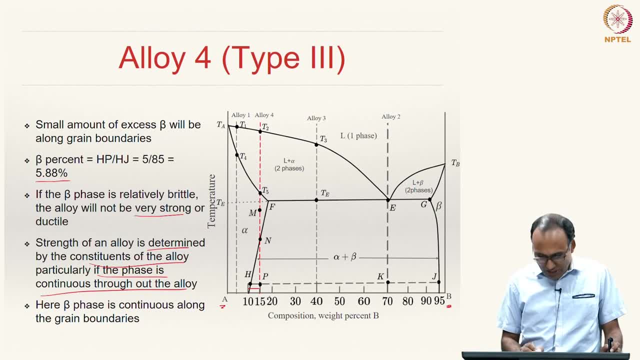 Particularly, if the phase is continuous throughout the alloy. and that is what happens particularly for alloy 4, because the beta phase will be continuous throughout, because the alpha everywhere has additional beta and the B additional B and that B comes out as beta and then it gets segregated there as beta phase and it is continuously distributed throughout the 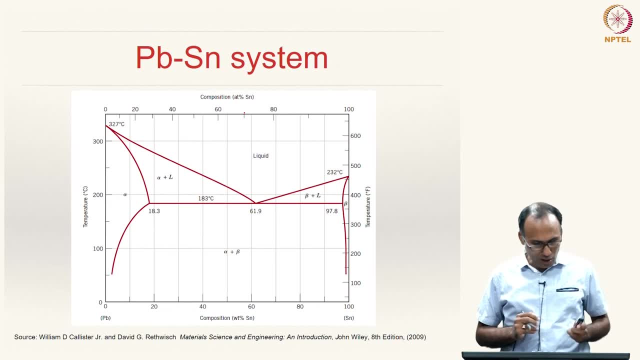 alloy. All right, So a real system? Yes, So a real system that has such a alloy phase diagram that we have discussed so far. 3 type of phase diagram is lead tin system, which is very well known to us as a solder, which 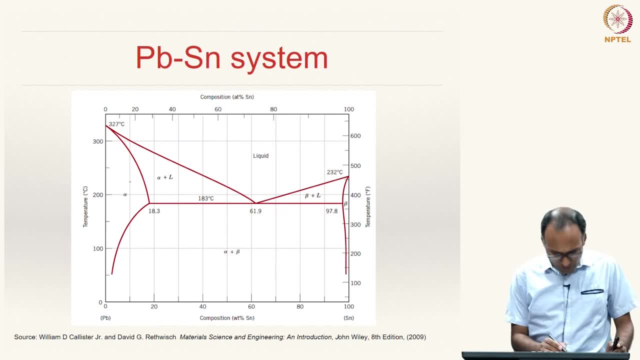 is used for solder joints. So here, alpha lead is on the left hand side, tin is on the right hand side, lead is soft and tin is known to be relatively harder compared to lead, and you have alpha solid solution and this is our beta solid solution. 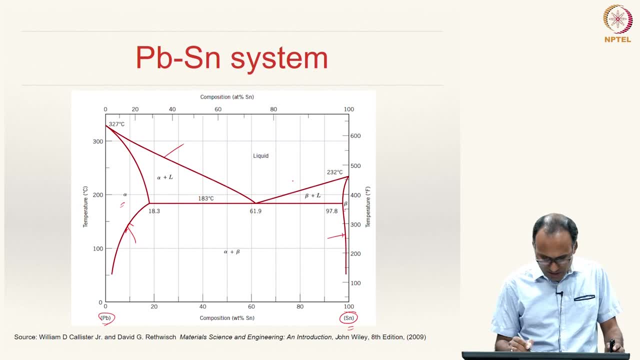 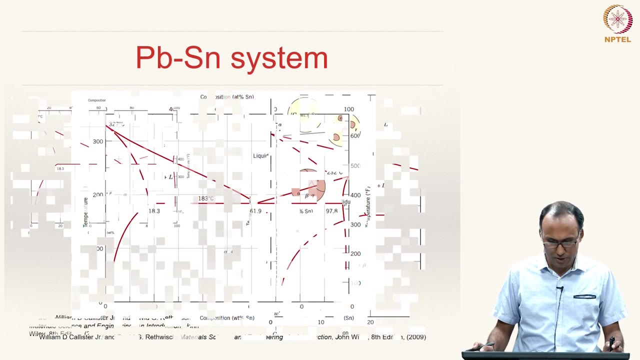 And this is our solvus line. these two are solvus lines and this is liquidus line and this is solidus line and that is our eutectic point right. So eutectic temperature is 183 degree Celsius and eutectic composition is 61.9 percent tin. 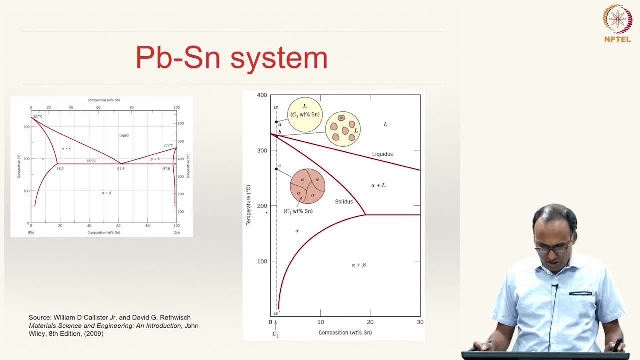 All right. So now again, if you look at the microstructures, the, it is like a, like a alloy, one that we have discussed. So you have liquid and then that will be forming in this two phase region. you will have alpha and liquid and by the time it comes here, you will have complete alpha right. 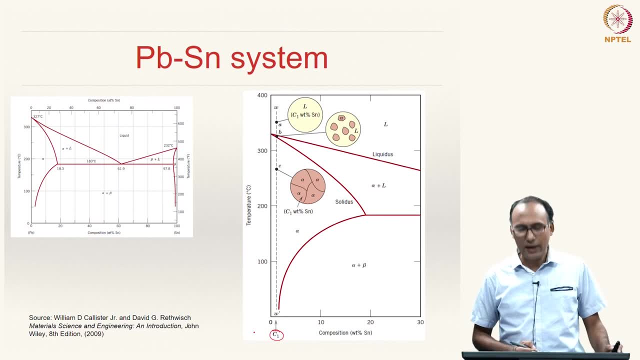 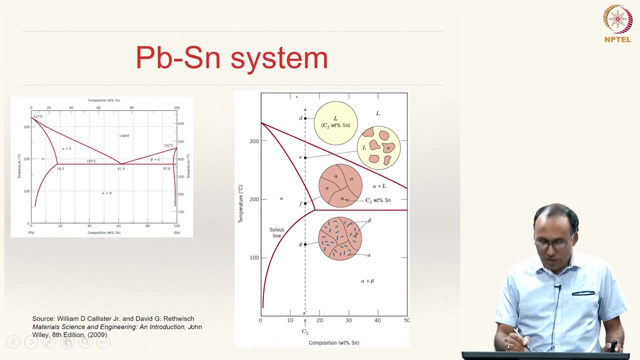 and the weight fraction will be, the composition will be C: 1 and it is a single phase region. it is exactly like our isomorphous system that we have looked at, And now this is the alloy 4 type that we have just now discussed. right, 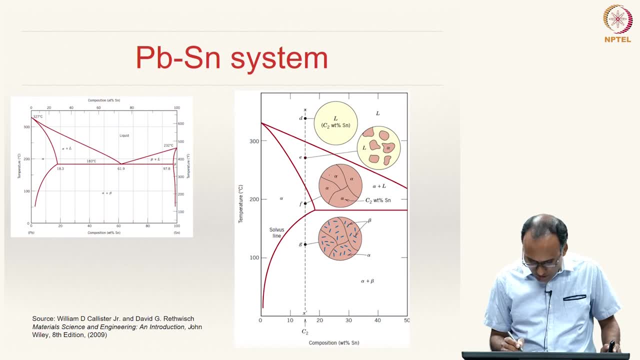 So you have complete liquid and then you are entering two phase region liquid plus solid. again you are entering pure solid- sorry, not pure solid- the single phase alpha, everywhere all are. So you have two alpha grains and by the time you cross this line you have over saturated. 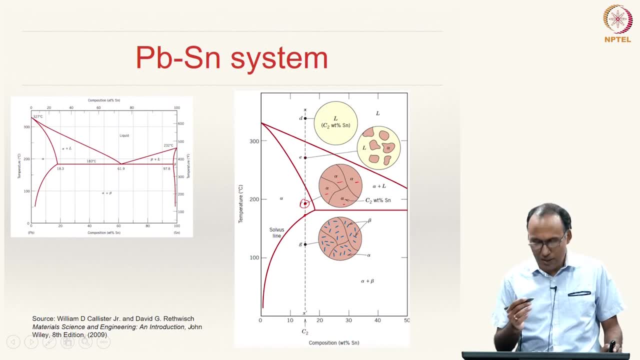 the over saturated alpha will have to give out B, but it cannot give B as pure B, but it gives out as beta and hence this beta phase is continuously distributed throughout the matrix. And if this beta phase happens to be a brittle phase, that can be detrimental for applications. 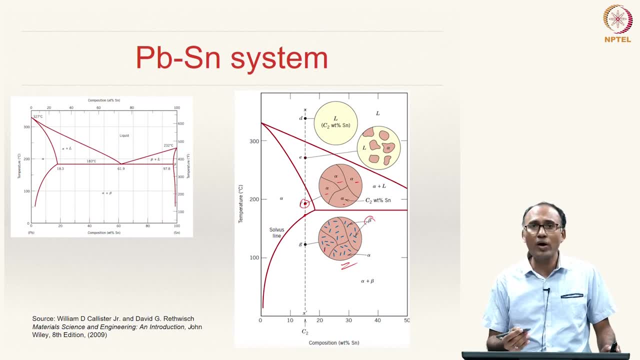 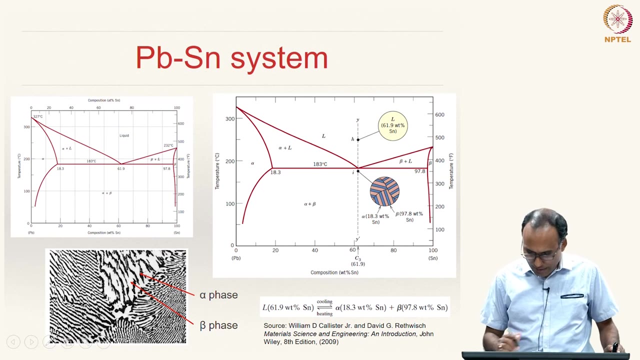 in which we are using this component and depending upon the nature of this beta, that the mechanical properties can be significantly engineered. And if you look at the eutectic composition, eutectic alloy, and again you have liquid, and at this point position, you will have formation of alternate layers of alpha and beta. 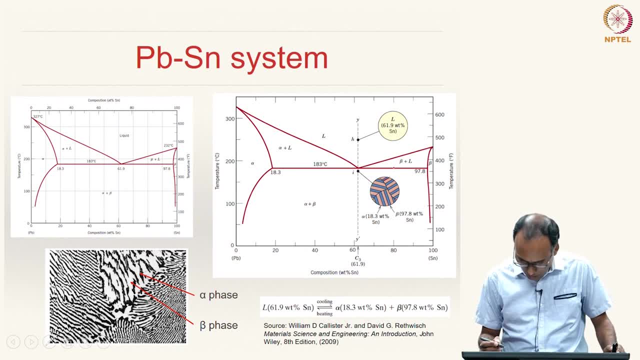 So here, the blue one is, let us say, blue one is beta and the pink one is alpha. so you have formation of alternate layers of alpha and beta. If you look the similar such a system under microstructure, microscope, you will see these. 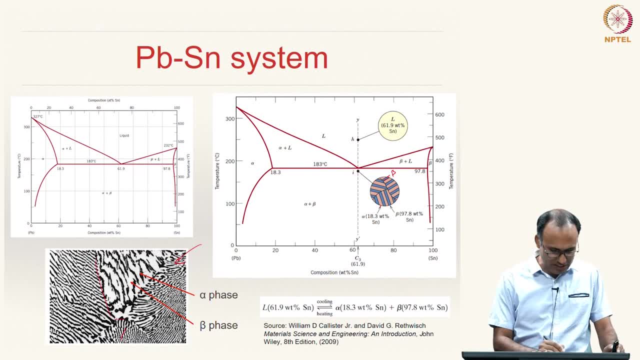 alternate layers of alpha and beta, and this is one grain and this is another: grain 1, grain 2, grain 3, grain 4,, all of them having these alternate layers of alpha and beta. So why these alternate layers of alpha and beta forms? 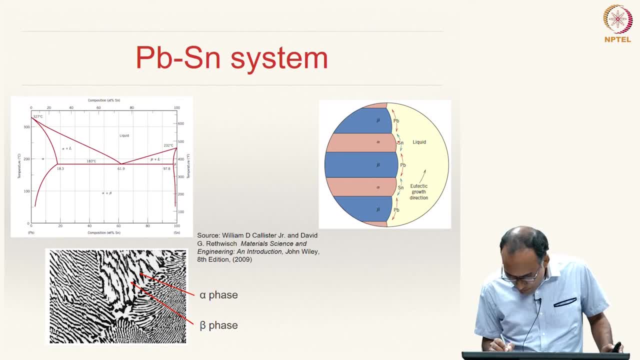 So, as we have discussed, let us say, a liquid here is actually having certain composition, and then that is solidifying. When it is solidifying alpha, the surrounding liquid becomes richer in beta or richer in B, and instead of forming this B elsewhere, it is much easier for B to travel to the neighboring. 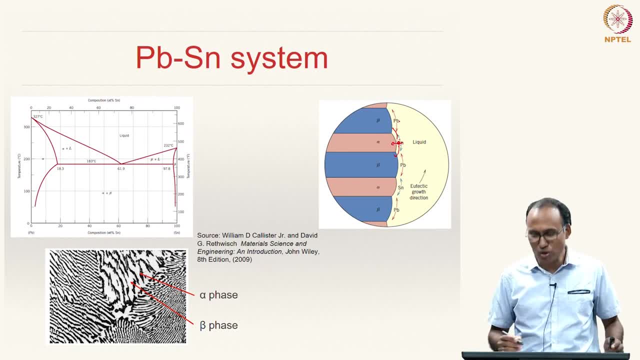 grains, That means the solid state, the atomic diffusion. if you are forming the alternate layers, the diffusion, atomic diffusion need to have, only need to take place only over a shorter distance, rather than forming individual grains a further away from each other. 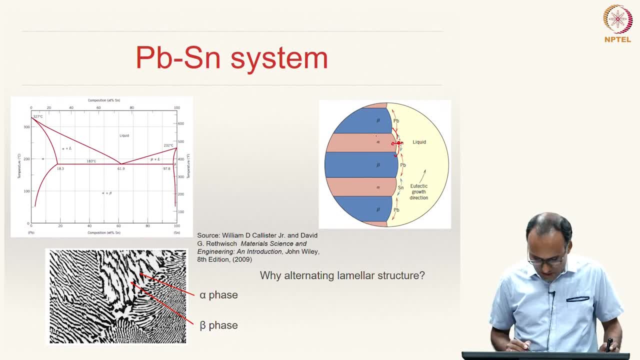 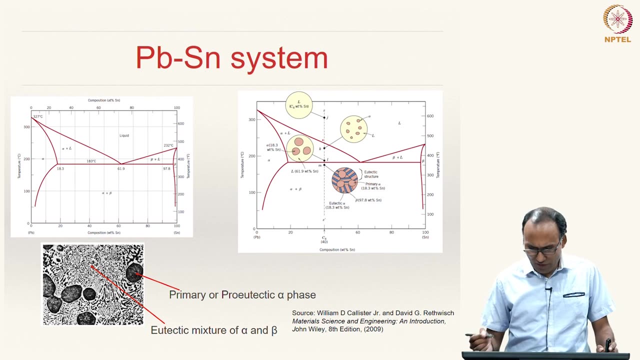 So the reason why the reason for this alternating laminar structure is because the atomic diffusion of lead and tin only need to occur over small distances if we are forming alternate layers. What happens? This is like our alloy type 2 that we have discussed so far, and you will have pro-eutectoid. 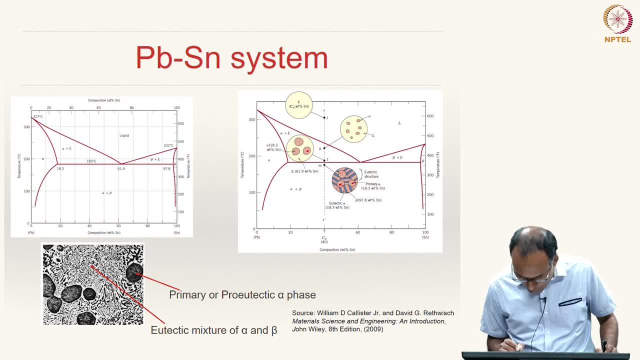 alpha. This is pro-eutectoid alpha and then, at this position, the remaining liquid, the yellow portion, will form alternate layers of beta and alpha. This is our beta and that is our alpha. So if you look at the microscope, you see this pro-eutectoid alpha and eutectoid mixture. 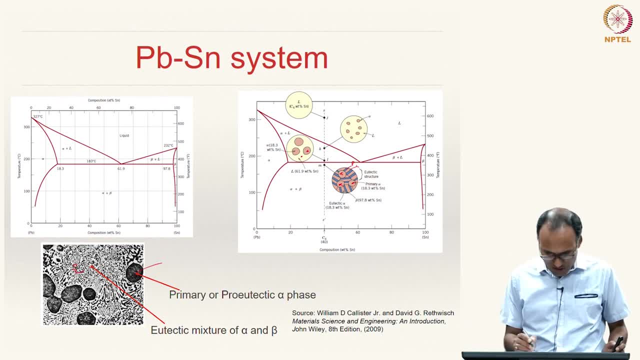 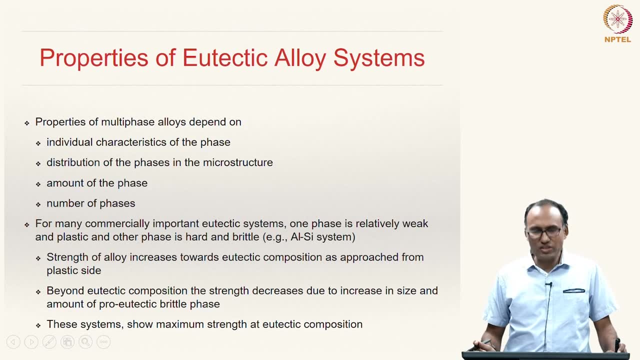 of alpha and beta and obviously you can calculate all the weight fractions by drawing the tie line and using the lever rule. So what are the properties of this eutectoid alloy systems? So the properties of multiphase alloys in general depend on the individual characteristics. 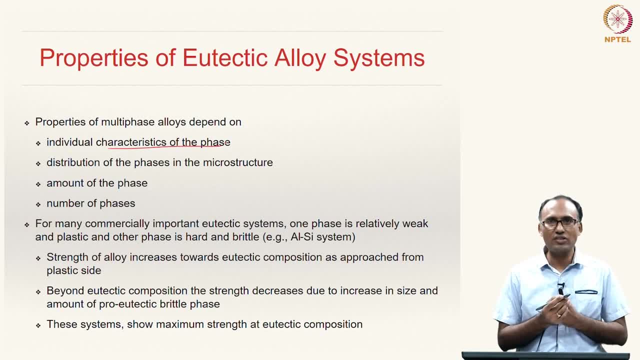 of the phase. What is the individual characteristics of each of these phases and the distribution of the phases in the microstructure, whether they are continuously distributed or not? If they are continuously distributed, what is the characteristic of the continuously distributed phase and so on, and what is the amount of that phase and the number of phases? 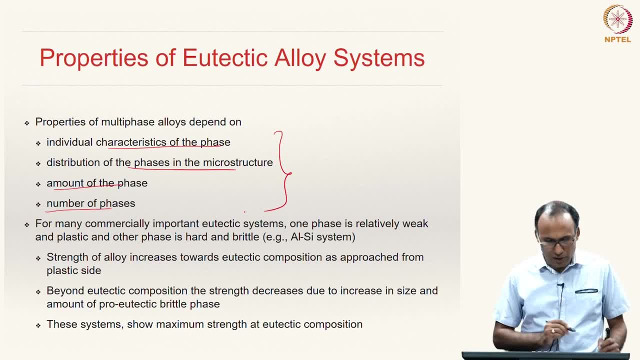 that are present. So these are going to determine the mechanical properties or in general the properties of the alloy system. So for several commercially important phases, For example in the mechanical phase, if the material is a little bit flexible there, 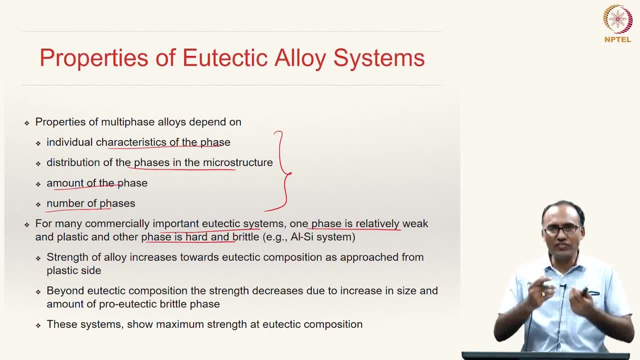 is a very high resistance to the surface moisture. So this is the resistance to the surface moisture. Now there are also many other phases of the process in the chemical process. So one phase is relatively soft and ductile, another is hard and brittle. a typical example. 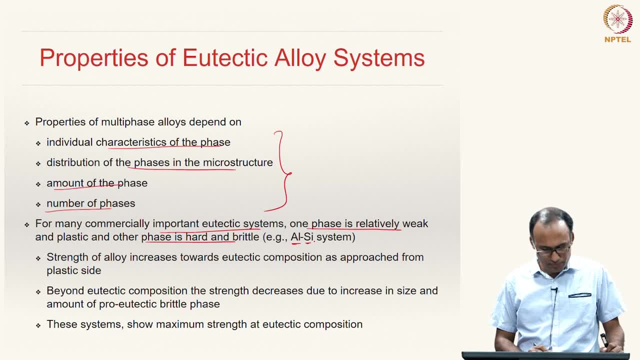 for that is aluminum silicone system. When we are dealing with this things- eutectoid systems- the strength of these alloys increases towards the eutectoid composition. So the strength of the alloy from pure metal-1 to pure metal-2.. 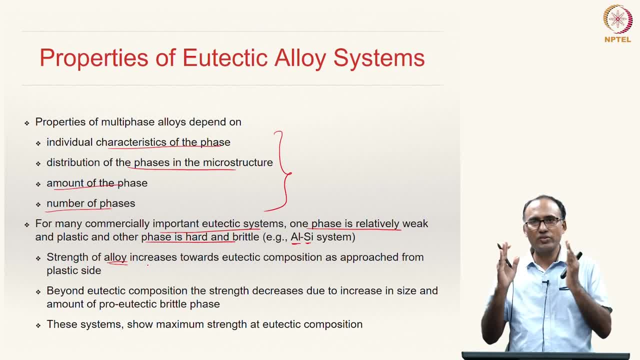 These alloys are very effective in the chemical process B and pure B. when you are reaching the eutectic composition from both sides. at the eutectic composition you usually have higher strength, So the strength of the alloy increases towards. 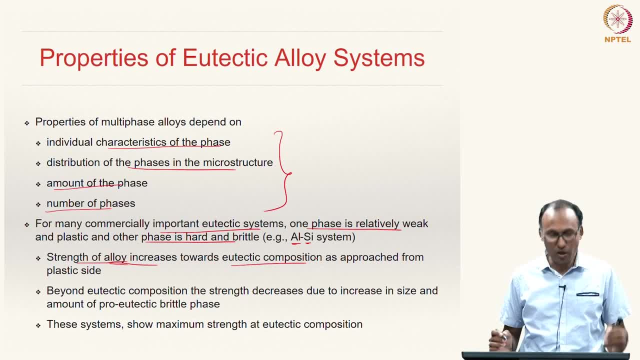 eutectic composition as approached from plastic side, not from the, as we are approaching from the plastic side, not necessarily from the brittle side. And beyond the eutectic composition, the strength decreases due to increase in size and amount of proeutectoid proeutectic brittle phase. Because the brittle phase is increasing, the 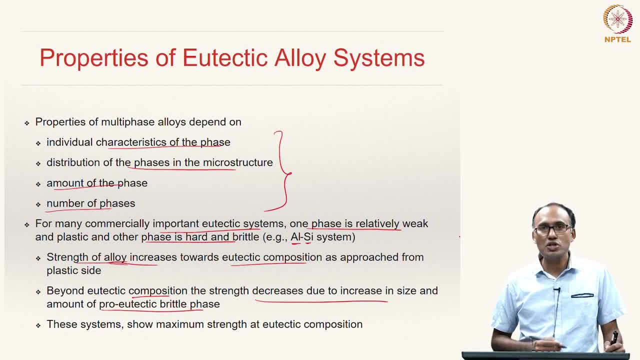 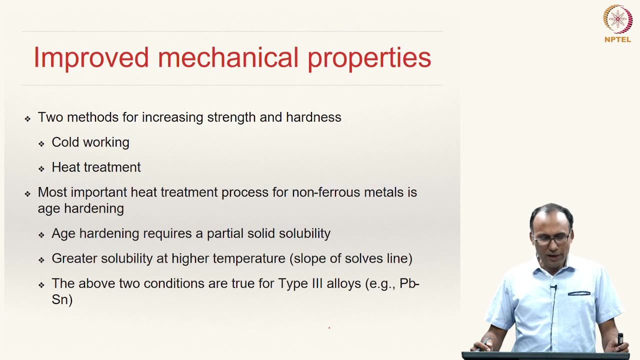 you will have reduction in strength And these systems show that means the eutectic system show a maximum strength at eutectic composition because after the eutectic composition if you have a brittle phase that is going to be detrimental for fracture. 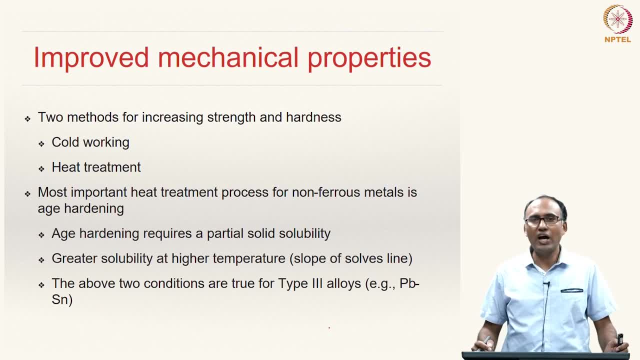 And how do we go about improving the mechanical properties if you have these continuous phases distributed throughout the system And then they are going to be detrimental to the mechanical behavior? So how do we go about improving the mechanical properties? So there are typically two methods. We can use cold working or that.